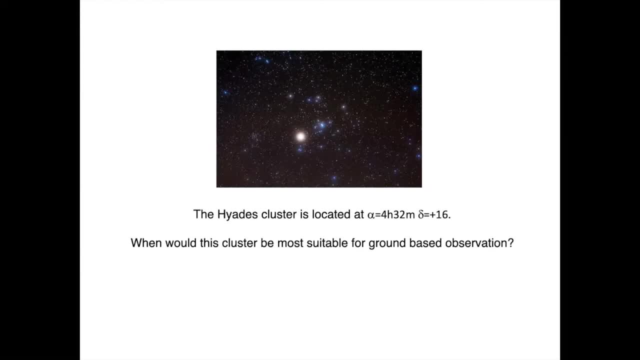 is just one of them. So let's start with the coordinates of a star. So as an example here, the Hyades Cluster right. The Hyades Cluster is located at right ascension 4 hours and 32 minutes and declination 16 degrees. 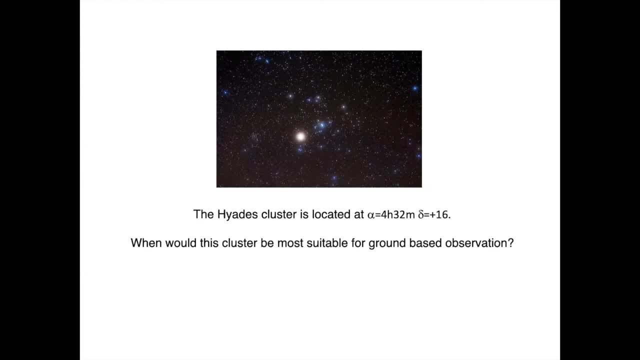 So a skilled astronomer knows from these numbers where in the sky the cluster is, what is the best time of the night to observe it, and what's the period of the year where it's going to be more visible. So when would this cluster be most? 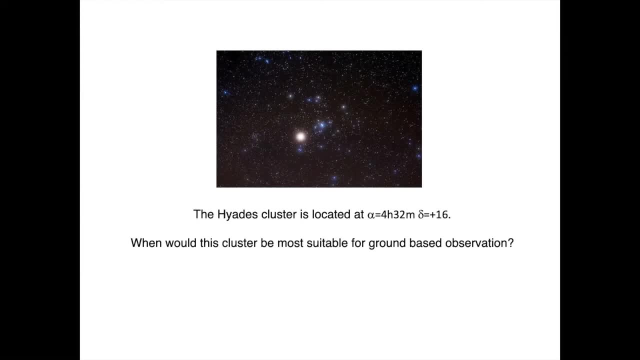 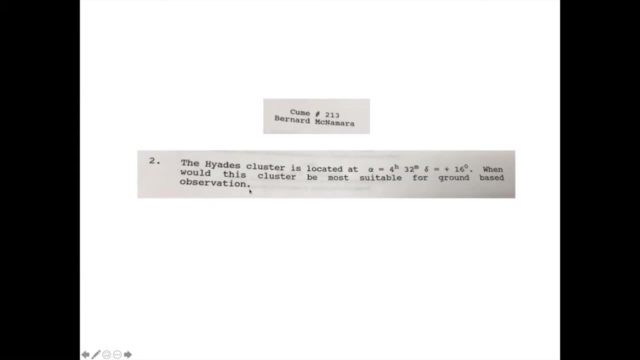 suitable for ground-based observation. When would it be most suitable for ground-based observation? That's a question. Actually, this question- and this is important- has been asked in a long, long, long ago, But you know, this is the kind of question that you can expect in an exam. 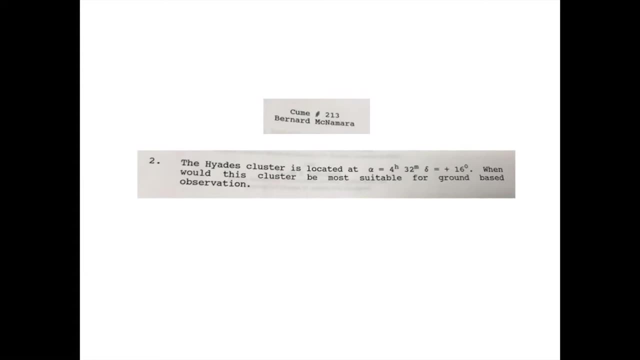 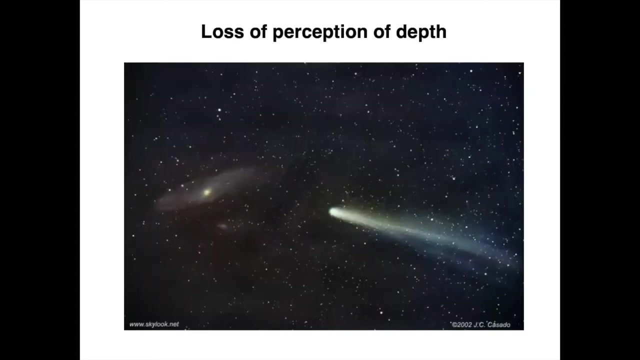 So, before we answer this question, let's start with the basics. When we look at a night sky, we are looking at stuff that is so far away that we lose the perception of depth. We're seeing here, for example, a comet and a galaxy on the same frame, right Of course, the comet and the galaxy. 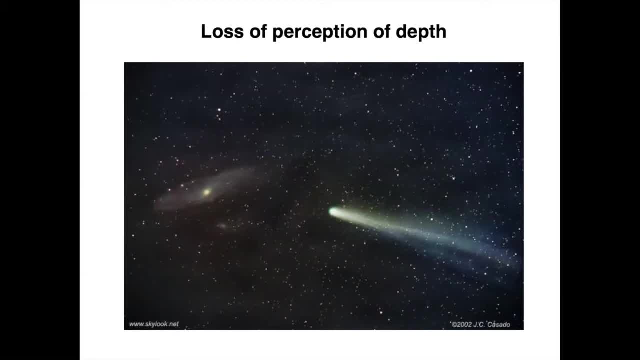 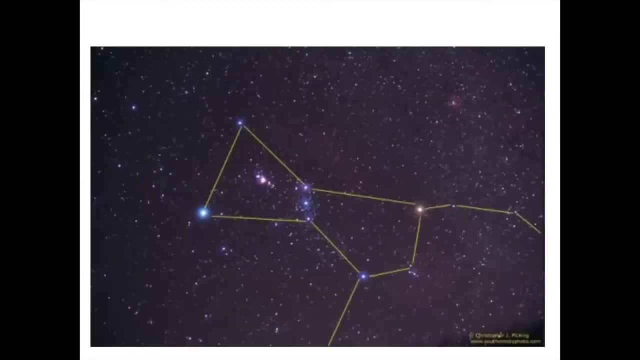 they're very, very far away. The comet is like on our face and the galaxy is like millions of light-years away. Still they look very close on the plane of the sky, and that's because we're losing the perception of depth, right? This is obvious also when we 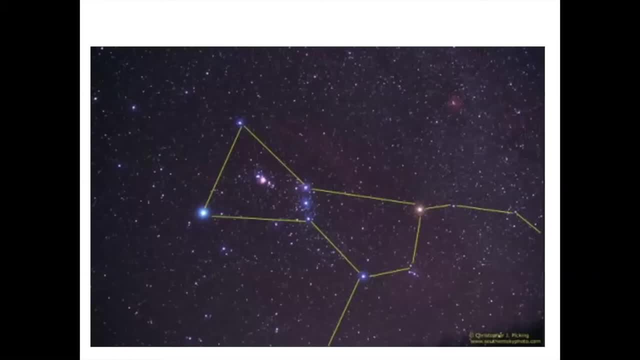 look at constellations. We grouped constellations because there are stars of similar brightness that look close to each other projected on the plane of the sky. But of course, in three-dimensional space- the stars, in a constellation, they can be very far apart. 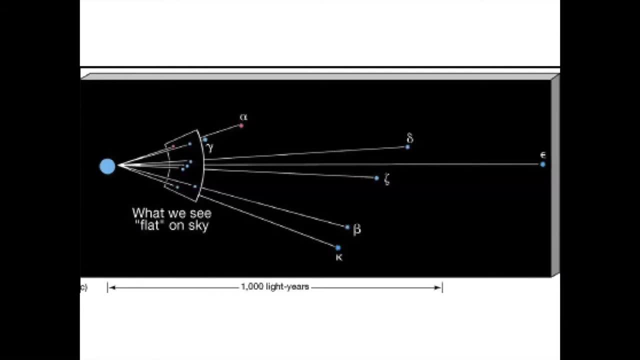 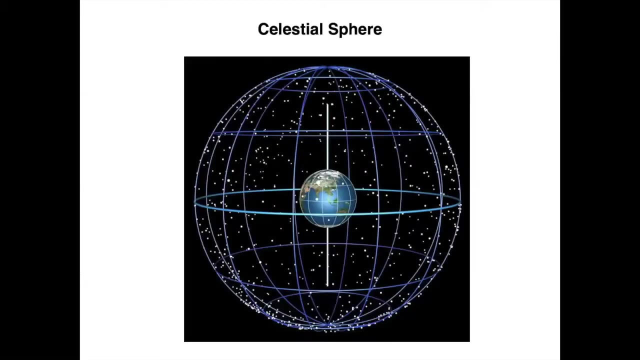 because we are losing this notion of depth, And in this third, in the third dimension, they may be very far away from each other If we lose this notion of depth. we see on the night sky all of these stars as if they were on the surface of a giant. 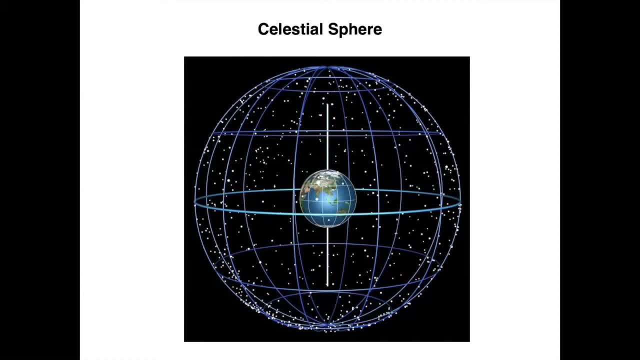 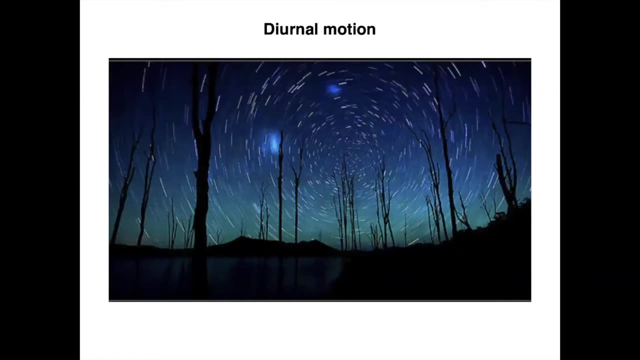 So we call this sphere the celestial sphere, And the motion of the celestial sphere is due to the motion of the Earth. That defines the diurnal motion right. This is an example of diurnal motion: The Earth is rotating and then, due to that, the stars are seen to rotate with the same. 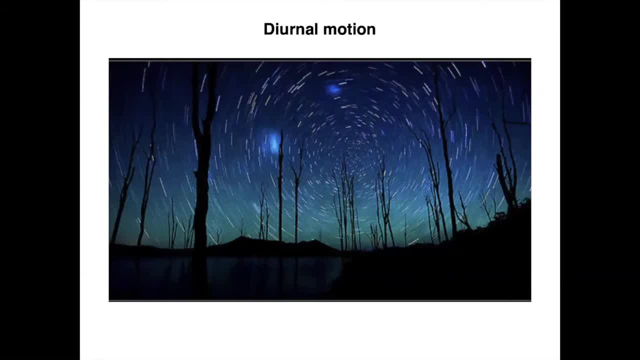 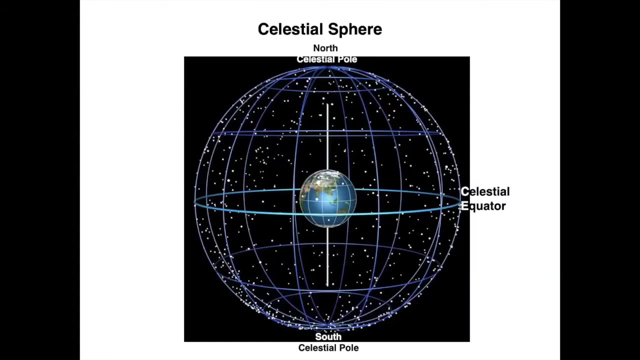 period of with the same period as the Earth rotates around itself. So we can start defining stuff on the celestial sphere And, the same way that on the Earth we have the equator and the poles, we can project these circles onto the celestial sphere. 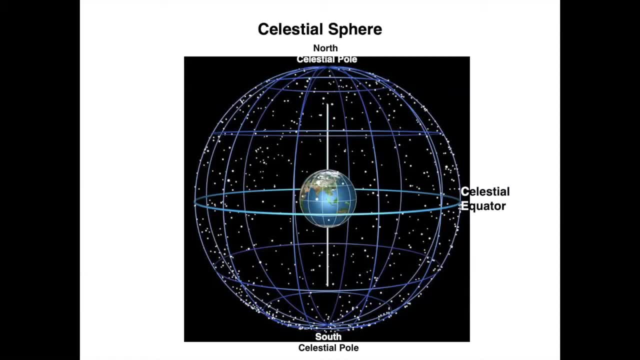 the circles at these points on the celestial sphere and we have the celestial equator and the north celestial pole and the south celestial pole. There, celestial equator is a projection of Earth's equator on the celestial sphere and the north celestial pole on the. 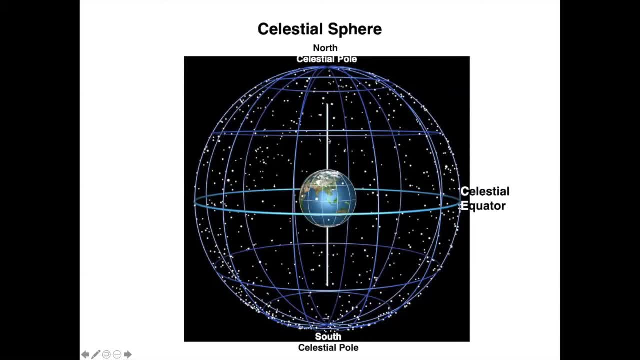 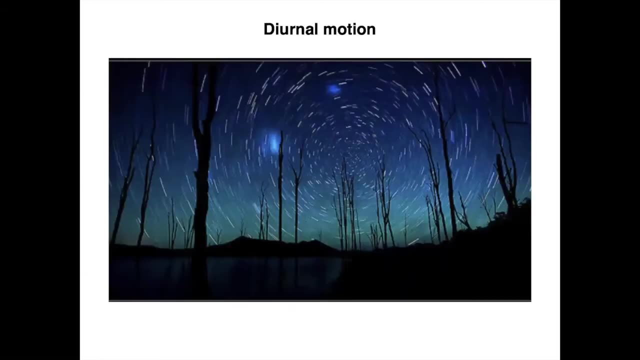 and the South Celestial Pole are the points where the projection of Earth's axis, Earth's rotation axis, meets the celestial sphere. The North Celestial Pole and the South Celestial Pole seem to be the points, then, about which the stars rotate around in their diurnal motion. 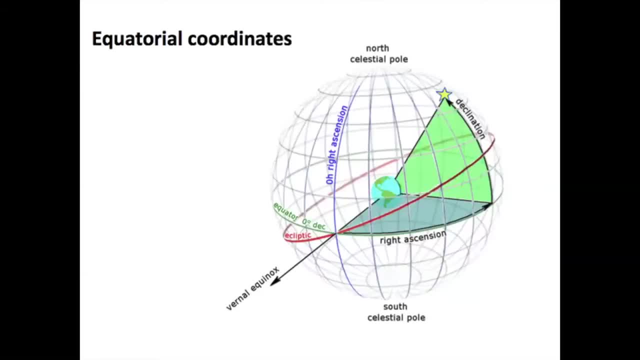 So that immediately defines equatorial coordinates. So the equatorial coordinates are one of the most used coordinates in astronomy And they are defined by these two quantities: the right ascension and the declination. So right ascension is the equivalent to what longitude would be on Earth. 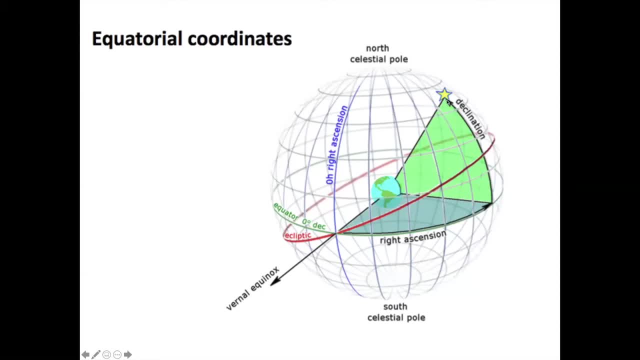 And declination is the equivalent of what latitude would be on Earth. So, in the same way that you can define a position on the surface of the Earth by giving the equatorial coordinates longitude and latitude, you can define a point on the celestial sphere. 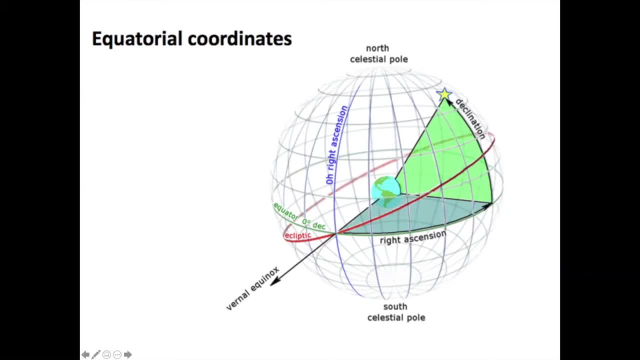 by giving right ascension and declination. The origin of right ascension is the vernal equinox And the origin of declination is the celestial equator For declination. that is natural because you have the equator as a bisection. 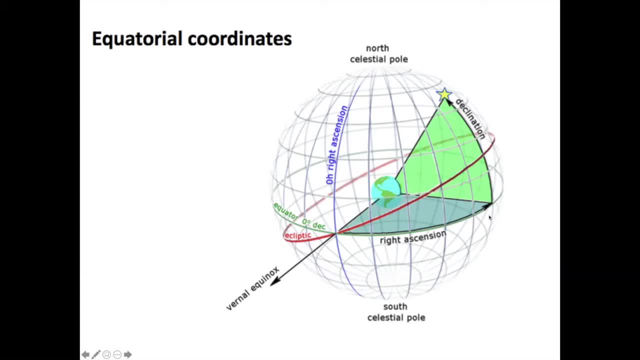 between the Northern and the Southern hemispheres of the celestial sphere, So it's a natural place to start counting declination For right ascension. you have to define a point In the same way that longitude on Earth is measured relative to the Greenwich Meridian. 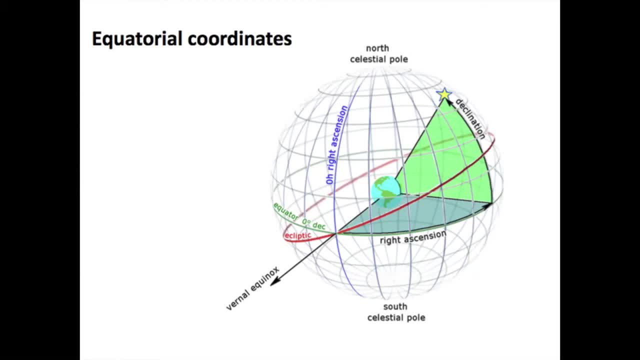 which is arbitrary. we needed to define an arbitrary point where we start measuring right ascension. This point was chosen to be the vernal equinox. Now, the vernal equinox is the intersection between two fundamental planes of the celestial sphere. One of them we already talked about is the equator. 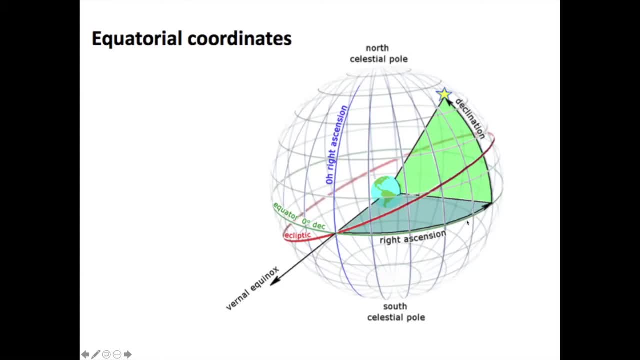 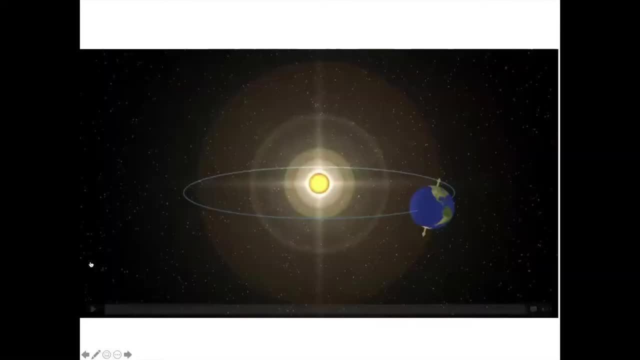 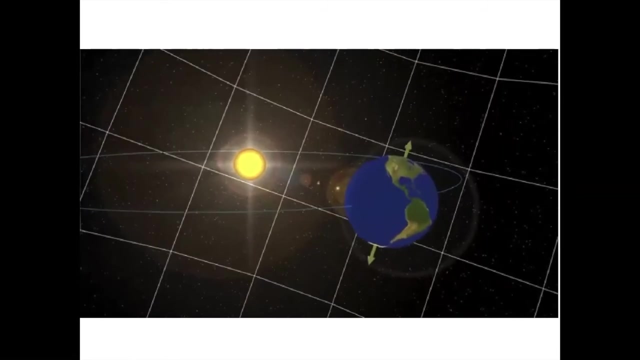 the celestial equator, the circle of zero declination. The other one is the ecliptic. Now, the ecliptic is the projection of Earth's orbit on the celestial sphere. So the Earth is going around in its orbit. So from our point of view, what we see is the sun moving. 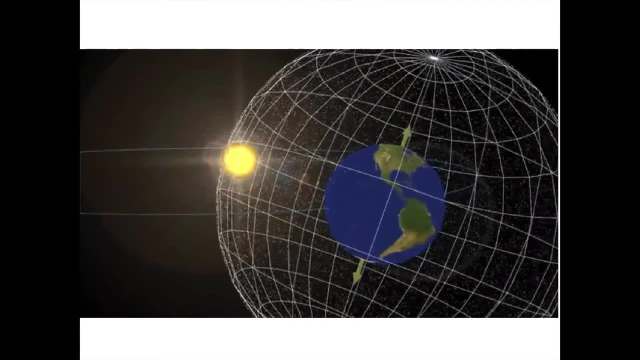 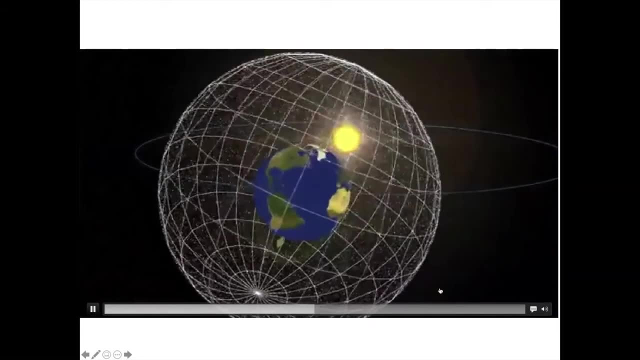 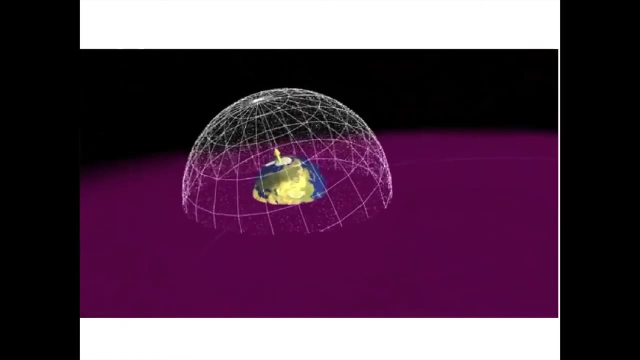 moving against the stars right. So we place that on the celestial sphere And what we're seeing here in this video is the position of the sun relative to the on the celestial sphere and where the plane of the orbit of the Earth. 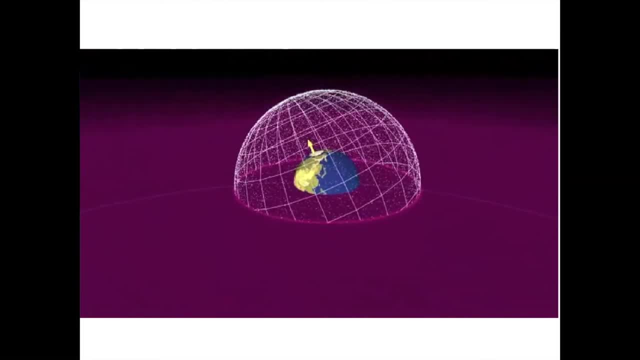 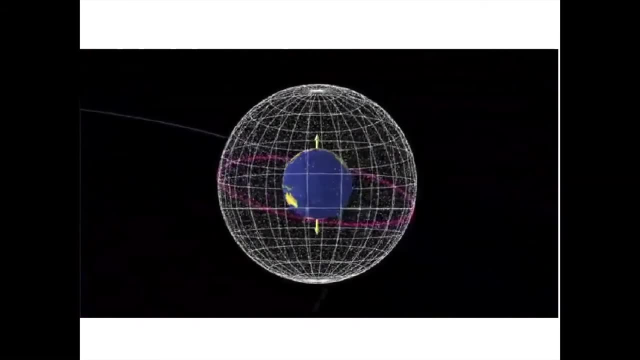 which is now this purple plane propagating all over intersects the celestial sphere. that's where you have the ecliptic. So that's a fundamental plane. From our point of view, the ecliptic is the path of the sun along the year in the sky. 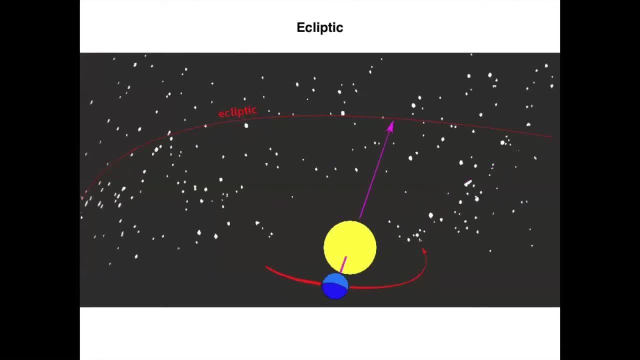 Here you see it's. of course it's us who are orbiting the sun right, Who go around the sun, But from our point of view, if you put on our reference frame, it is the sun that is moving. 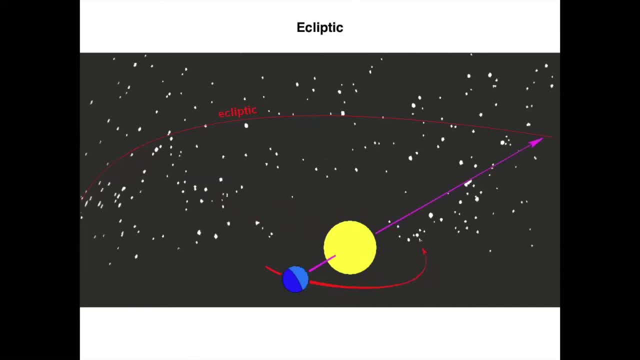 So the motion of the sun against the background, the distance, the orbit, the sun, the ecliptic, and the sun, that's the distance starts- describes the ecliptic. So here you have the solar path in equatorial coordinates. 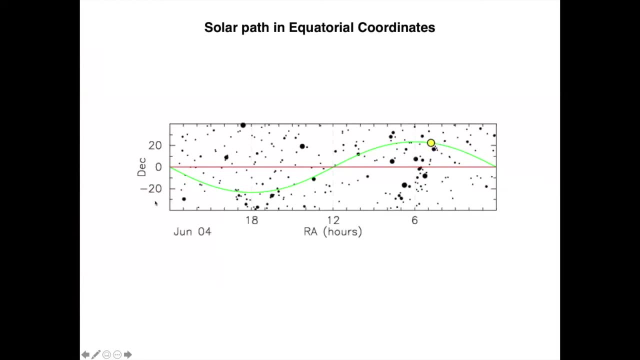 Is the motion of the sun here in right ascension and declination. So the sun first goes up, Right up in declination, reaches a maximum point, stars to go down, goes back here to the celestial equator that finds an equinox. 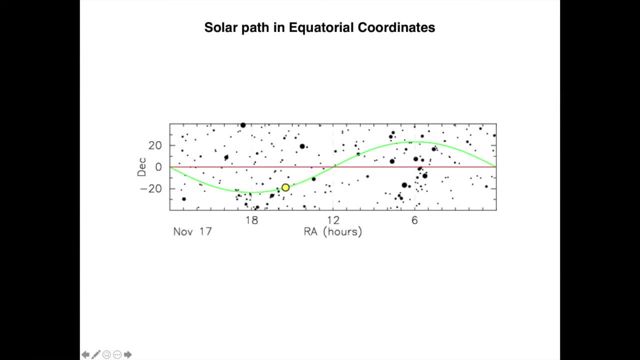 and then goes again at 18 hours of red ascension. That's the maximum south declination. And then it goes up again towards the equator. So this point here on the equator, that's the vernal equinox, It's the beginning of spring. 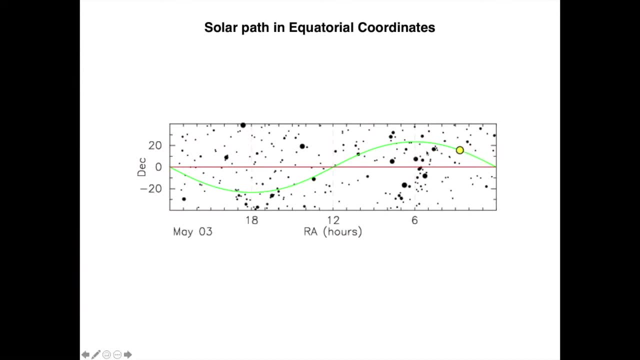 That's why it's called the vernal equinox. The other points here, the maximum point, this is the summer solstice in the northern hemisphere, when the sun is at its northernmost point, And then it goes again. that's the fall equinox. 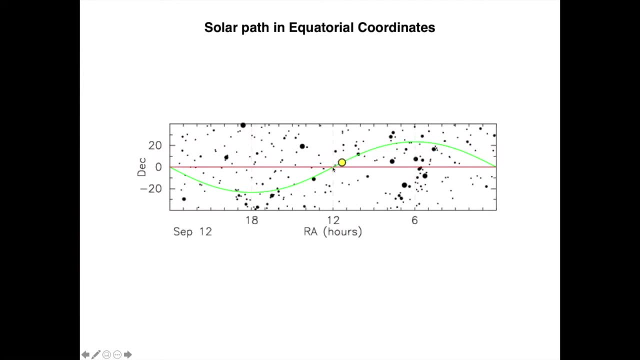 the September equinox on the northern hemisphere And then here in December, that's the winter equinox. the December equinox, winter in the northern hemisphere and summer in the southern hemisphere, And after that going back then to spring. So the intersection between the equator and the ecliptic. 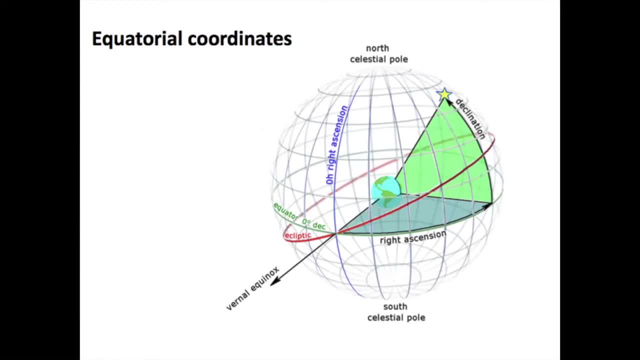 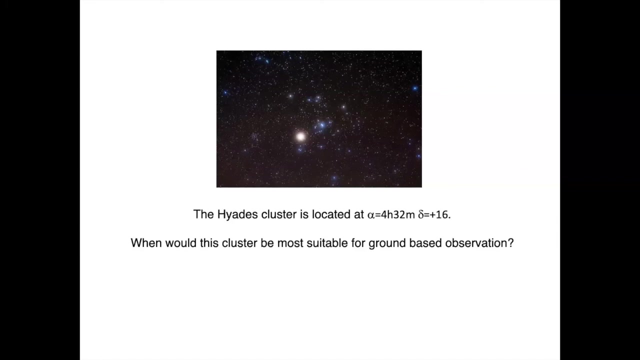 defines two points. These points are the equinoxes. There is the vernal equinox and the alpine equinox. The origin of right ascension is the vernal equinox by definition. So, based on this knowledge, we can already answer the question back from the cube. 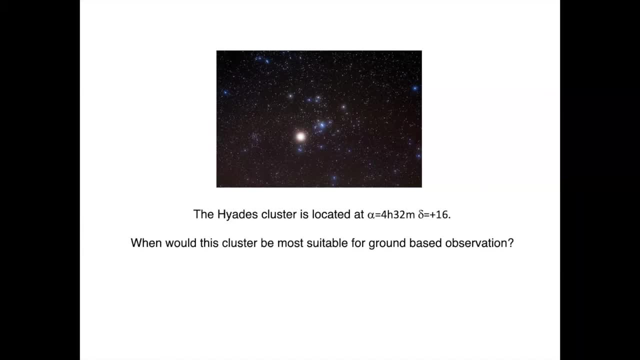 The height of this cluster is located at alpha, equal to four hours and 32 minutes. alpha is the right ascension and delta the declination is 16 degrees. When would this cluster be most suitable for ground-based observation? In fact, to answer this question, 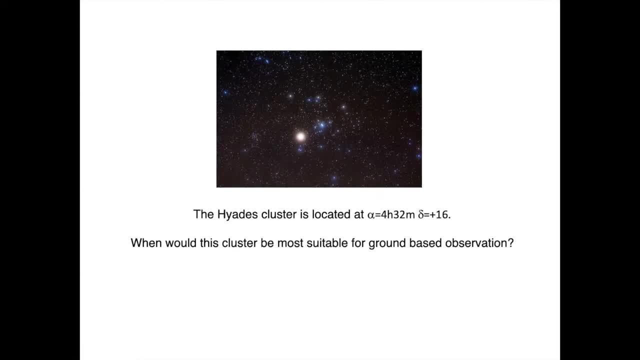 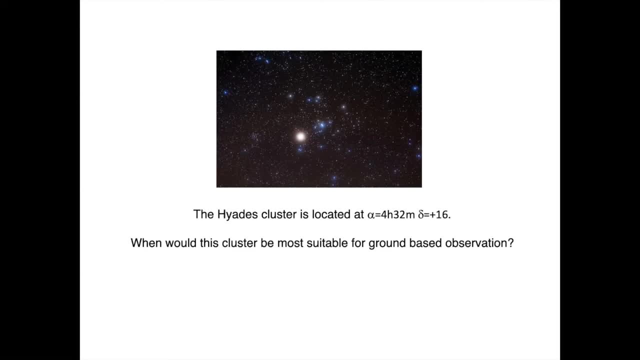 So you want to have the sun as far away from it as possible. The sun should be diametrically opposed to the location of the star cluster. That means that the right ascension of the sun should be 16 hours and 32 minutes. 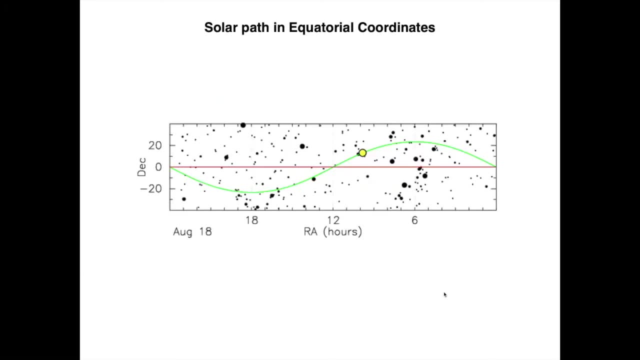 That would be on the opposite side of the sky, so it's visible all night long. So we can go back here to this plot, to this image, to this animation that is showing the path of the sun along the year, and follow here on the x-axis. 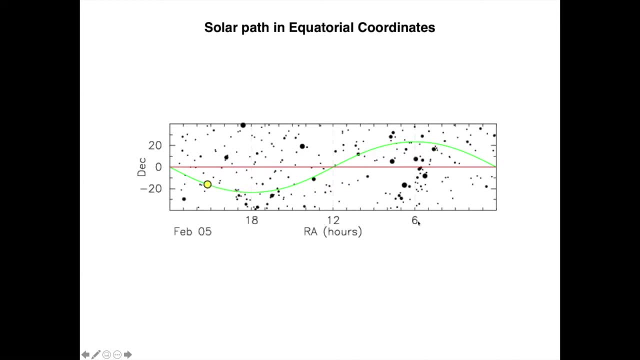 the path of the sun. So the star cluster is around here, right Four hours and 30 minutes of right ascension according to the x-axis. You want to know when the sun is going to be at 16 hours and 30 minutes.